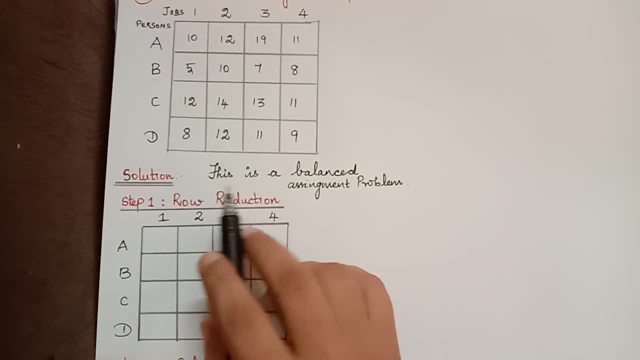 That is, we have to subtract the minimum entry of each row by the number of columns. So if the number of columns is equal to the number of columns, then it is an unbalanced assignment problem. If the number of columns is equal to the number of columns, 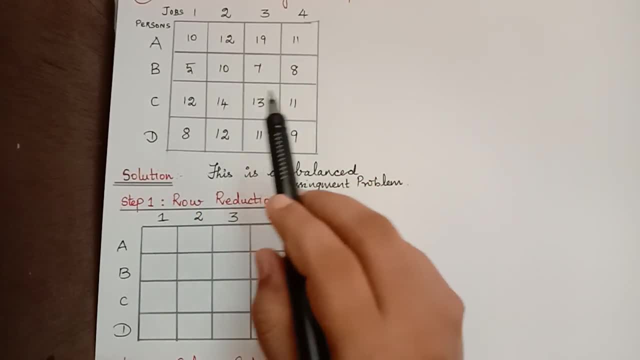 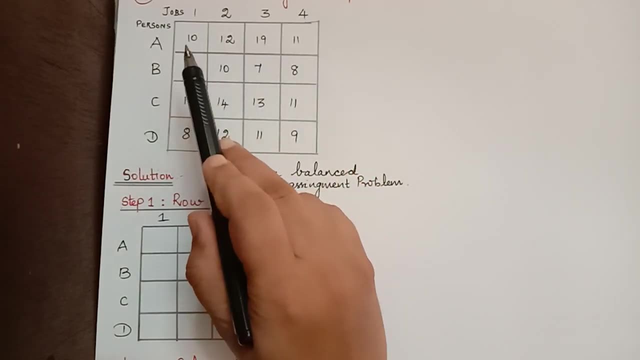 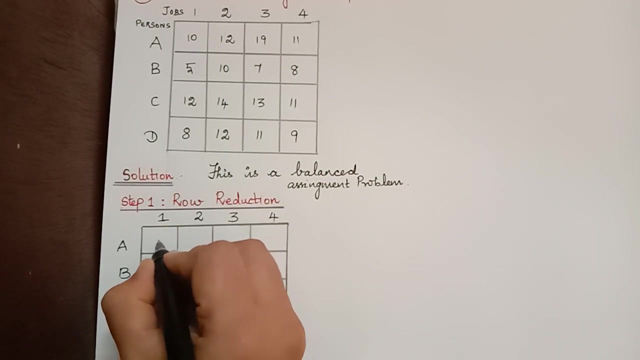 from all the entries of the respective row in the cost matrix. Now if we see in this problem, in the first row the minimum element is 10.. Now we have to subtract 10 from all the elements of the first row. So 10 minus 10 will be 0,, 12 minus 10,, 2, and here it is. 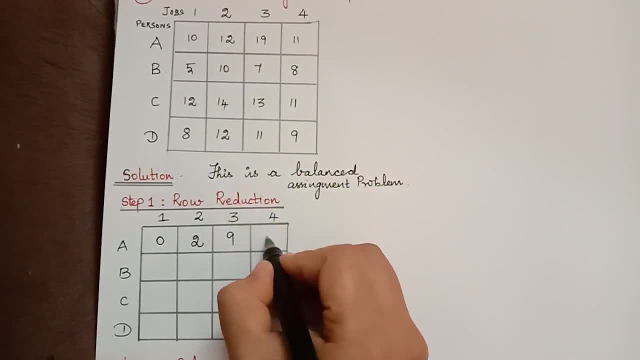 19 minus 10,, so 9 and 11 minus 10, it is 1.. Similarly, the minimum element is 10 minus 10,, so 9 and 11 minus 10, it is 1.. Similarly, the minimum element from second row is 5.. So. 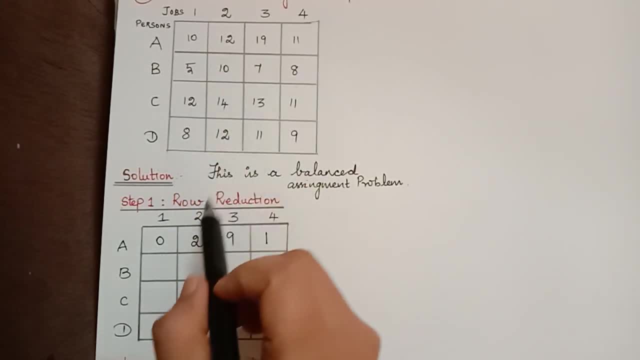 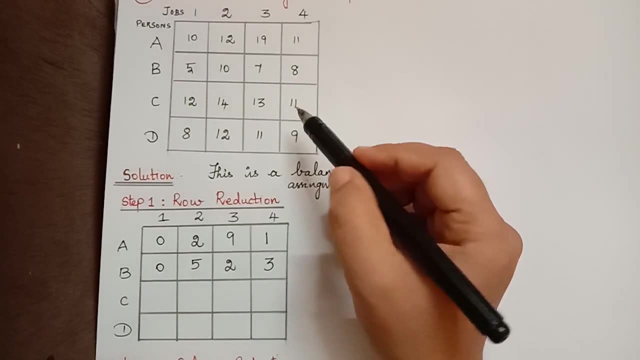 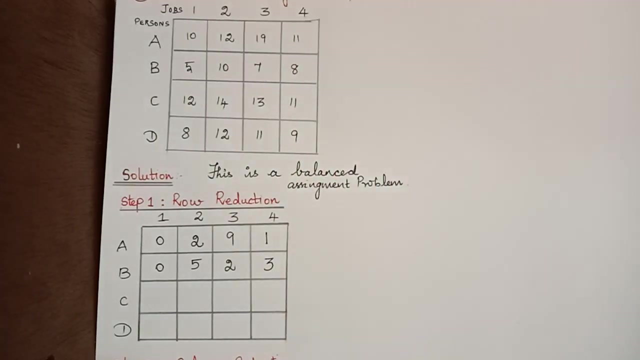 if we subtract 5 from all the elements of this row, we get 0,, 5,, 2,, 3.. The minimum element in the third row is 11.. So we have to subtract 11 from all the elements. So 12 minus 11 is 1, and 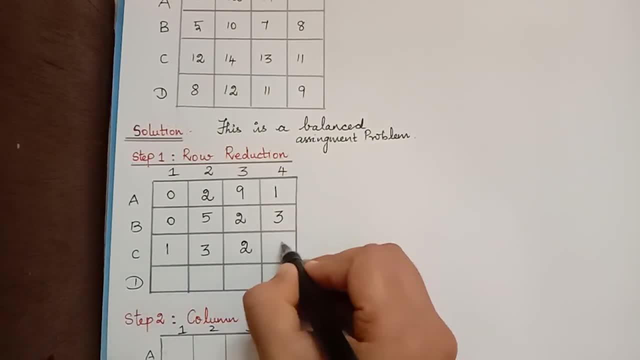 here it is 3, here 2 and 0.. Similarly, the minimum element in the third row is 11.. So the minimum element of the last row is 8.. So 0,, 4,, 3 and 1.. Next we have to move on. 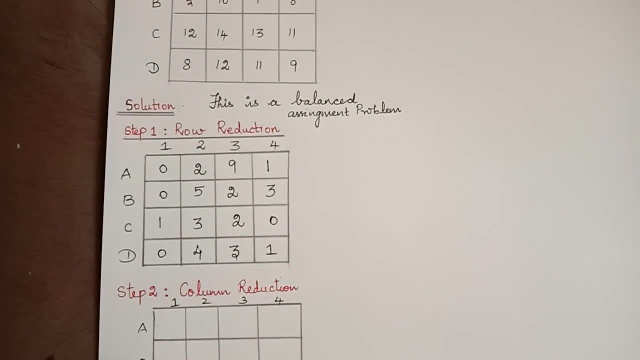 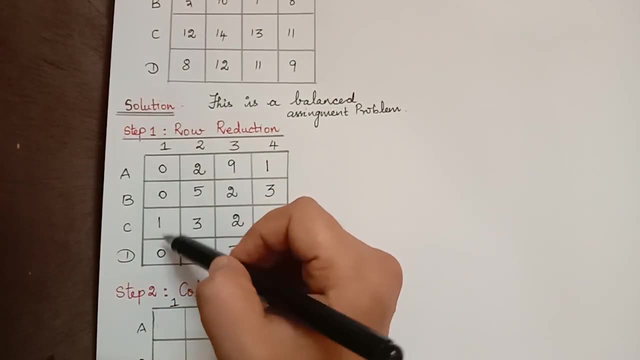 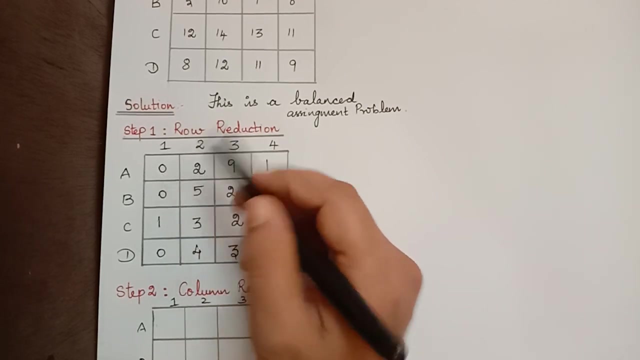 to the next step, which is column reduction. So in this we have to consider the matrix that we have obtained in step 1.. Now we shall consider the first column. The least element of this column has to be subtracted from the other elements. The least element is 0. So 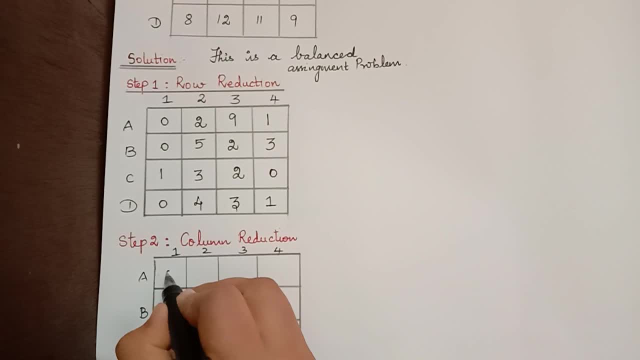 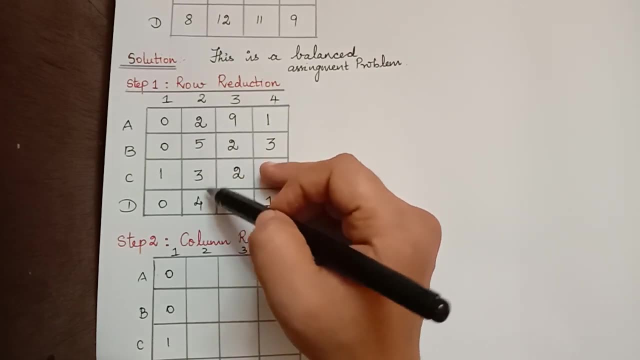 we have to subtract from the other elements. So we have to subtract from the other elements. So we have to subtract 0 from all the elements and definitely we will be getting the same column to be repeated. Now if we see in this, the minimum element is 2.. So we have to subtract 2. 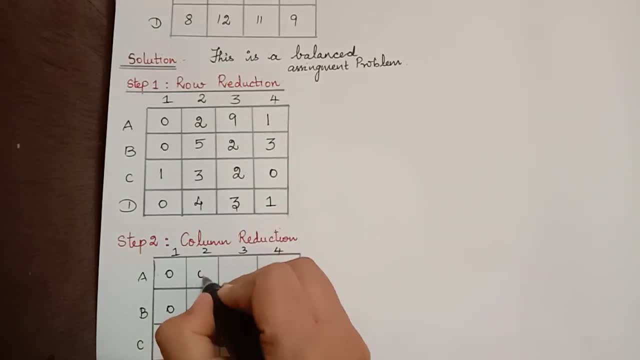 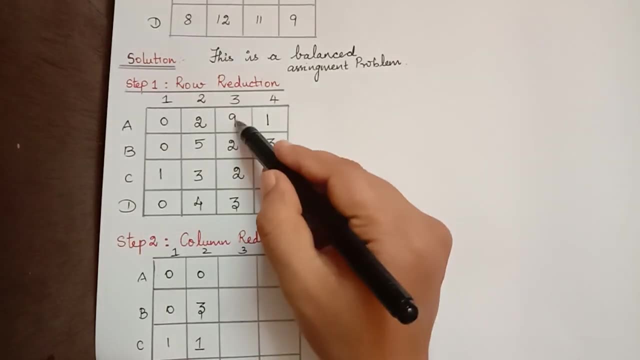 from the each element of this column, So 0,, 3,, 1 and then 4 minus 2, which is 2.. The least element of the third column is 2.. So we have to subtract 2 from all the other elements, So this becomes: 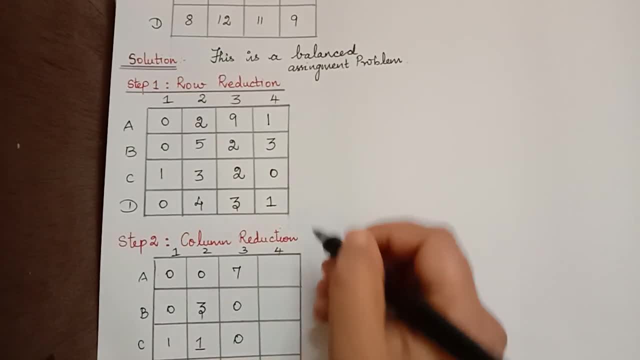 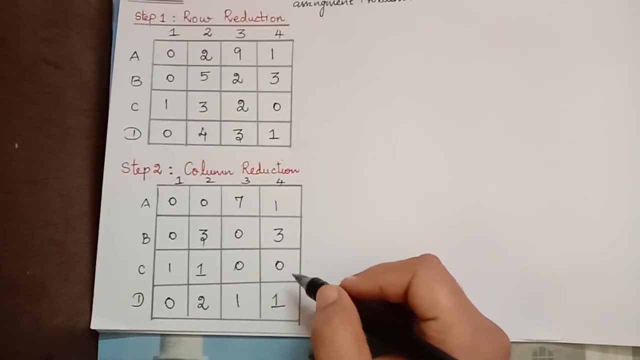 0, 0, 1, and here, the last column, the minimum element is 0. So obviously, 1 minus 0 is 1, 3, 0 and you get 1 over here. Now we have to go to step 3.. So that is, we have to start. 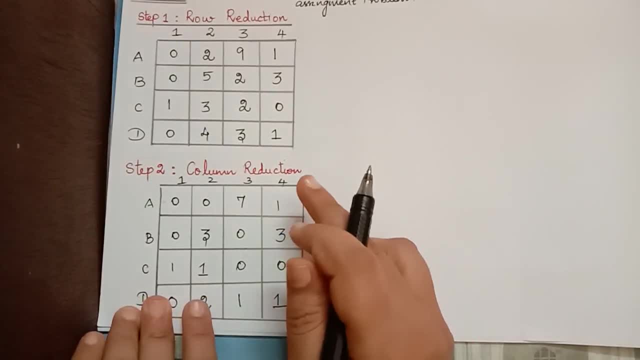 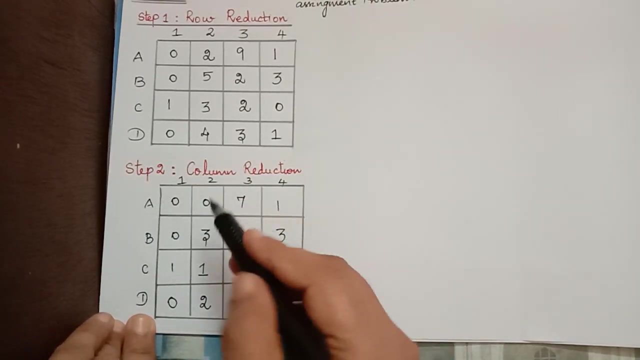 with first row of the matrix received in this step and we have to start examine how many 0s it has. Now the idea of the problem is each job has to be assigned to a one person. So now we have to check. we have to check that each row and column has one 0. And so 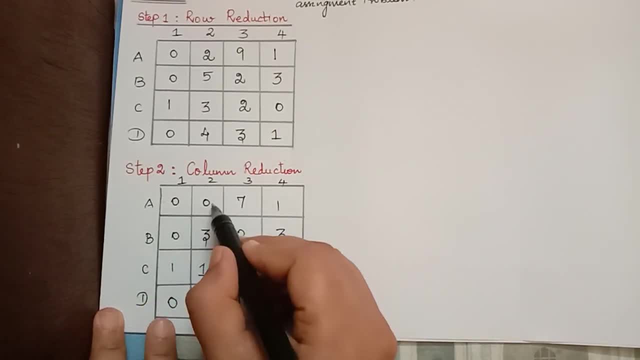 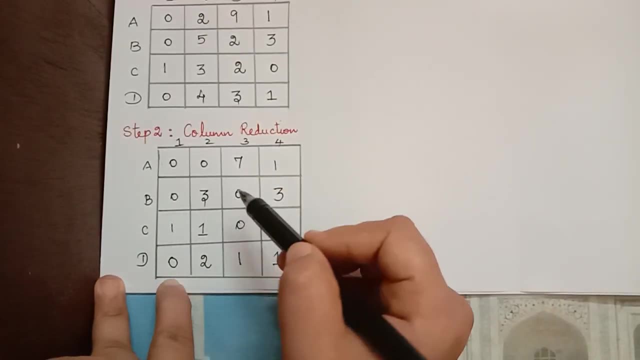 if we see in this row there are two 0s, So let us not select any of the 0.. Now here, also in this row, again we have two 0s, So we shall move on to check. 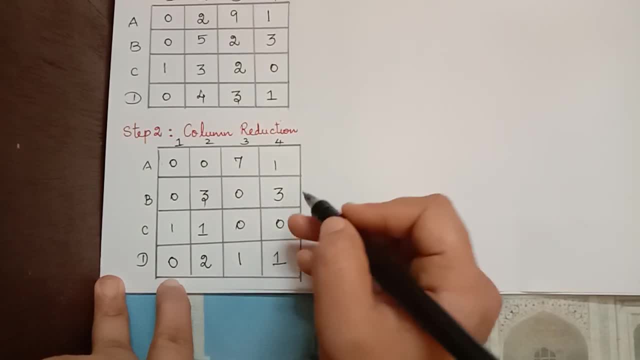 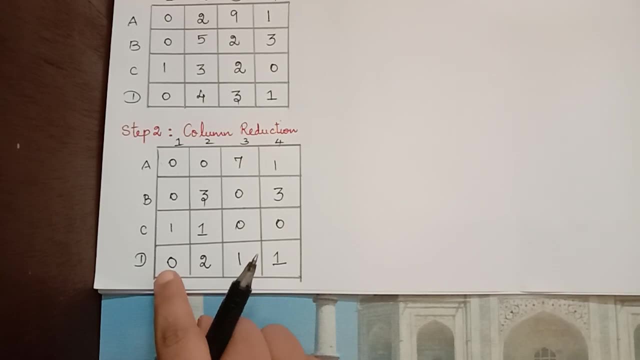 So here also we have two 0s and so we shall move on to the last row. So if we can see that in the last row the only 0 available is this 0.. So definitely we have to select. 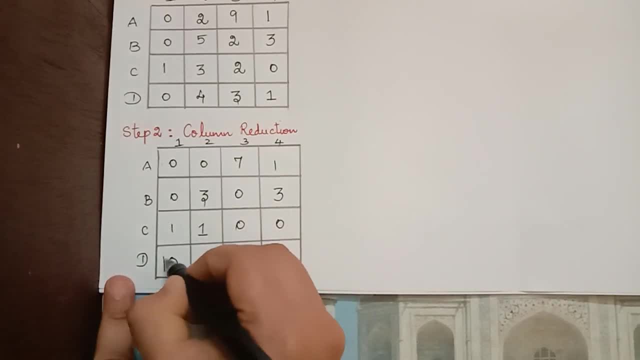 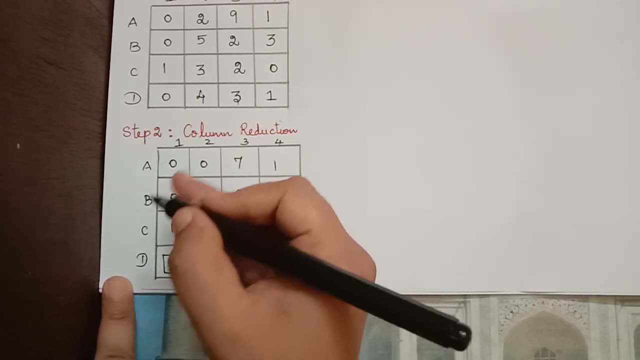 this 0 for this row. So we shall select this 0.. So once we are done with that, we have to strike out the corresponding 0s of that column. So after selecting this, we have to strike out this 0.. So after selecting this, we have to strike out this 0.. So after 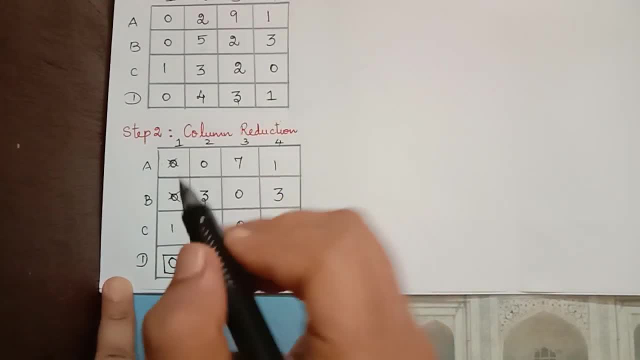 selecting this, we have to strike out this 0 and this 0.. Now again, we have to proceed with the same procedure. We have to check the first row, how many 0s it has now. Now this 0 has been stricken off, So it has only one 0. So definitely, that 0 has to be selected. 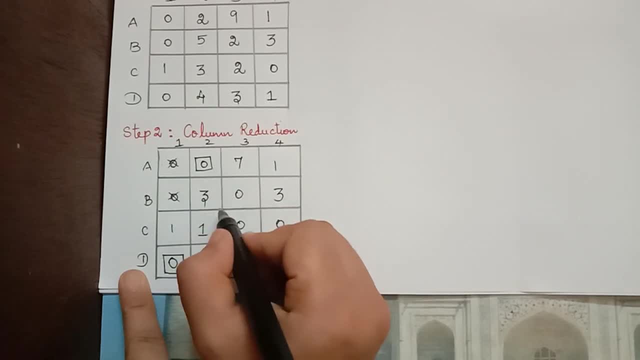 for this row Now. next, we shall move on to the next row. Now again, this row has this single 0.. So this has to be selected. Now, because we have selected this 0, this, we have to check out the corresponding column.